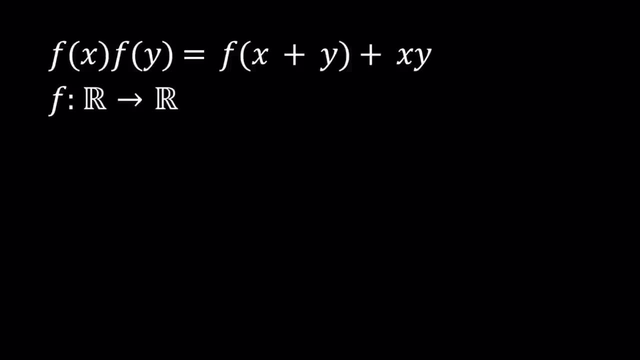 Hello everyone. In this video we're going to be solving a functional equation from BMO 2009.. BMO stands for British Math Olympiads. All right, great, So let's go ahead and take a look at this equation Now. functional equations are kind of fun. Don't get frustrated, because sometimes they. 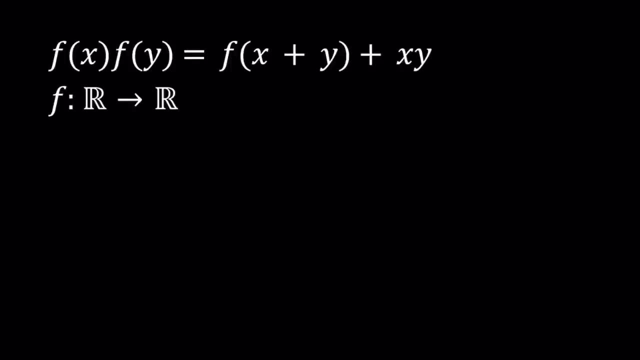 look complicated And this one is probably could be considered an easier one. Anyways, we have f of x times f of y on the left hand side and we have the f of x plus y plus xy on the right hand side, So we're going to be finding the functions that satisfy this, And f is defined from real numbers. 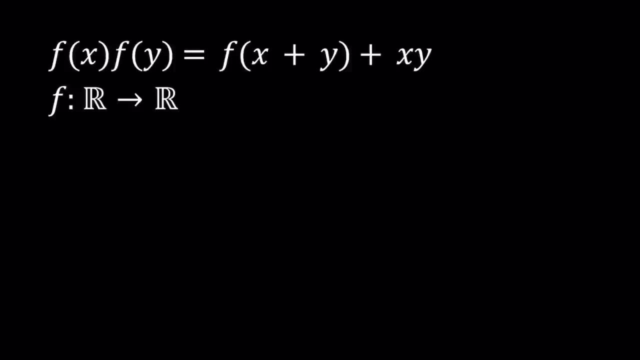 to real numbers. Great, So we're going to start- and this is kind of like a general strategy for most functional equations. We're going to start by replacing x or y with zero, because f of zero plays an important role in functional equations. 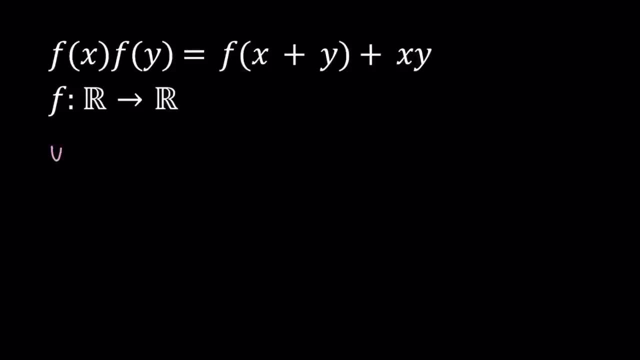 So let's go ahead and replace y with zero, And then this gives us f of x times f of zero, equals f of x plus zero, which is f of x, And then this becomes just plus zero. The reason why I wrote zero is because I'm going to subtract f of x, So you can kind of see that zero is going to be left. 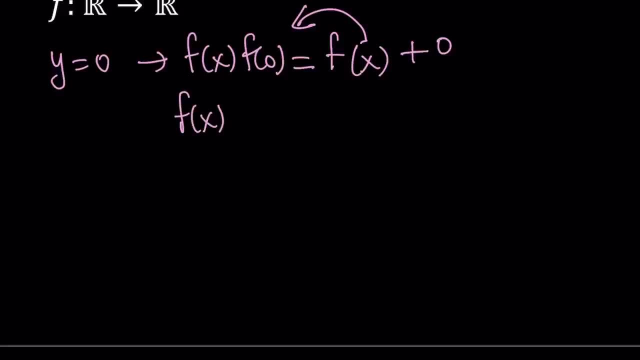 over on the right hand side. So this is going to give us f of x times f of zero. minus f of x equals zero. Awesome. Now my goal is to find f of x, but I'm not going to find it from here. 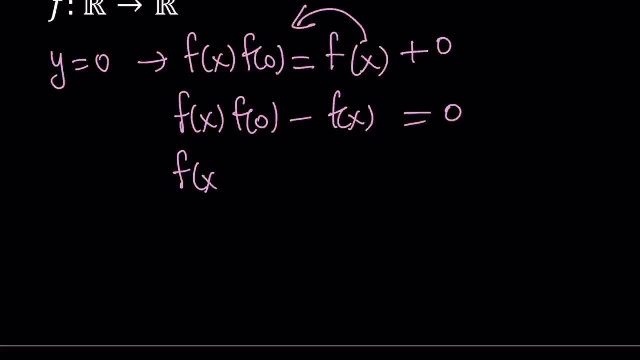 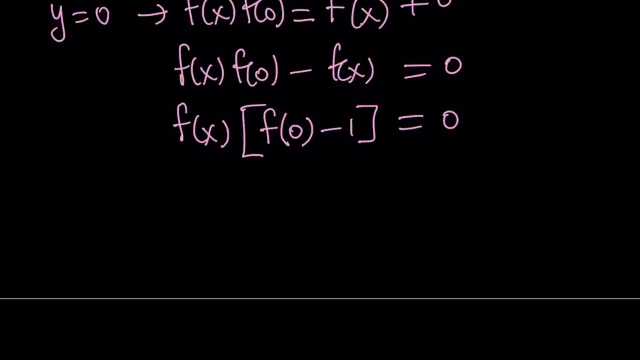 but I'll find some useful information. So let's go ahead and take out f of x, because f of x is a common factor, And inside the parentheses we find f of zero minus one equals zero. You know, zero product property. when you have a product that is equal to zero, either factor can be zero. 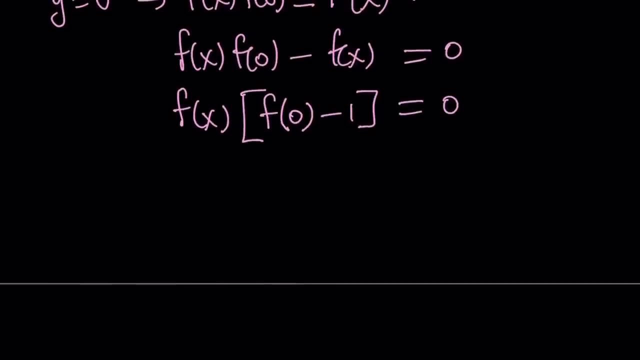 It can be both as well, but we don't know. We have to each case. So from here we get two possibilities. Either f of x is zero. But when I say f of x equals zero, I'm not talking about a particular value, but more like it's equivalent to zero. 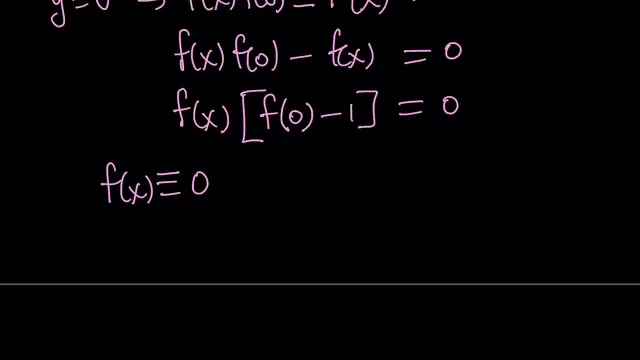 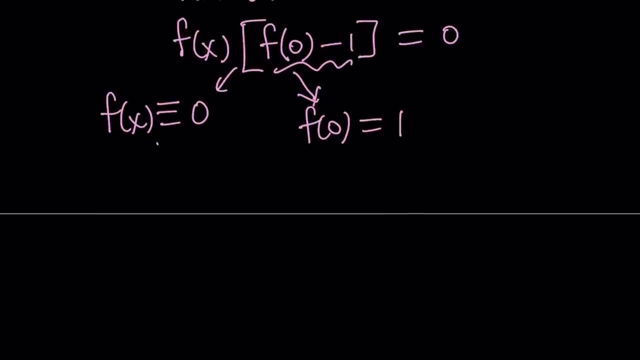 So it's kind of like a zero for all x values. And then the other possibility from here is f of zero minus one equals zero, And this means f of zero equals one. So at least one of these has to be true. But here's the problem. The first case is impossible. And why is it impossible? Let's 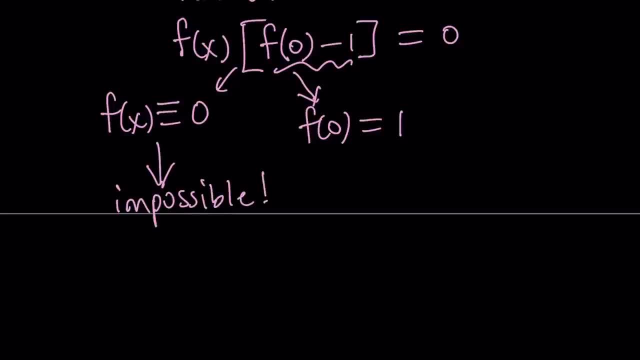 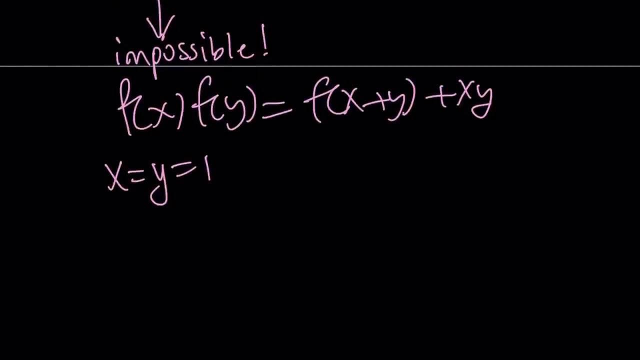 take a look at that. In the original problem- remember it was f of x times f of y equals f of x plus y plus xy. If you replace x and y with one at the same time- because it's from reals to reals, you can pretty much use any value here- you're going to get f of one squared equals. 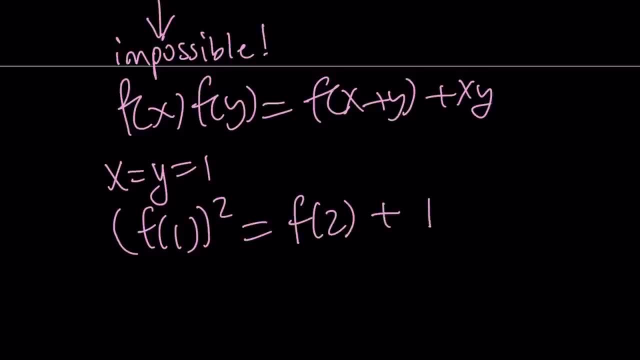 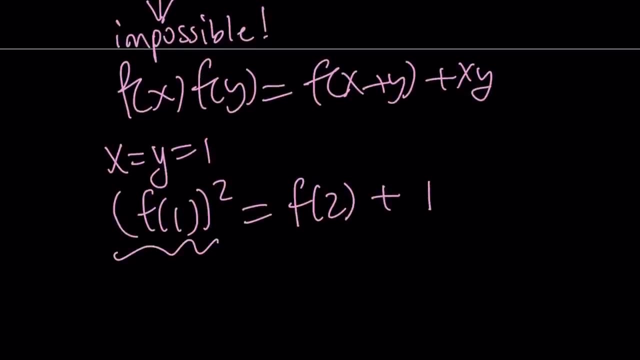 f of two Plus one. Now, if f of x is identically zero, then you're going to run into a problem, because this is going to be zero And it's going to be zero. but zero equals one. That's not true. So 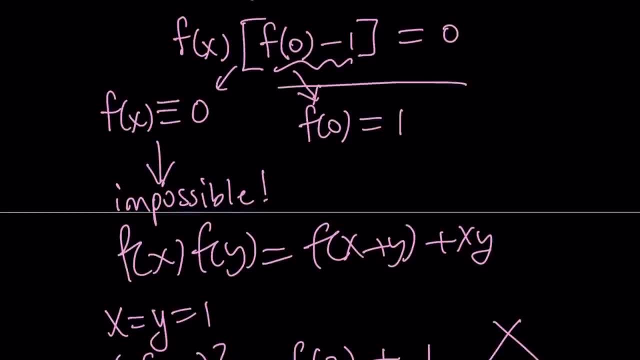 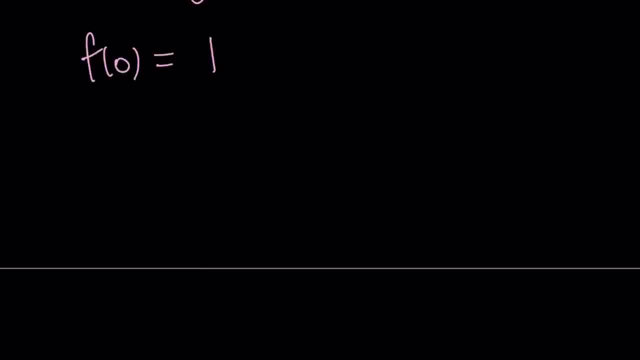 the first case scenario is not going to work. Therefore, we have to go with the second one, which means f of zero equals one. All right, awesome. This is a good finding. Let's go out and hold on to it And let's see what we can do next. So now. 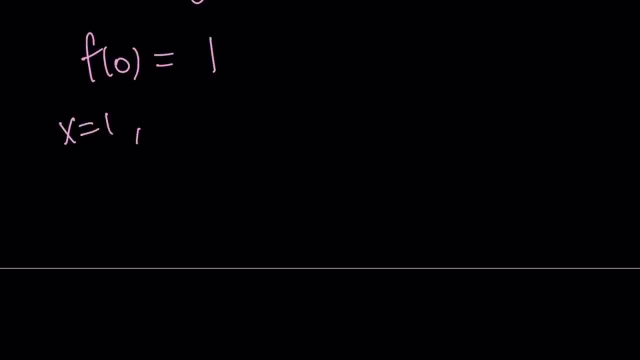 in the original equation. I'm going to replace x with one and y with negative one. Hopefully you have a copy of the original, because I don't really want to write the equation every time, Not because I'm lazy, but it's kind of boring, I guess. So, anyways, replace x with one and y with. 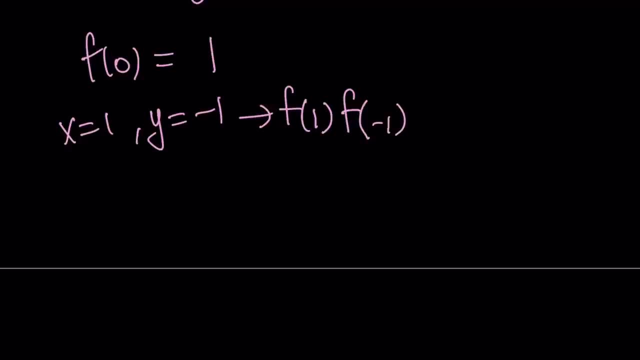 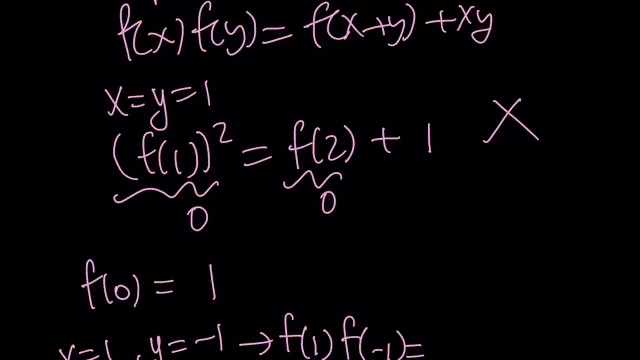 negative one, you get f of one times f of negative one equals. Now if you look at the original problem, you're going to notice that you get inside the parentheses here: in f of x plus y, you get f of zero. So that's kind of like. 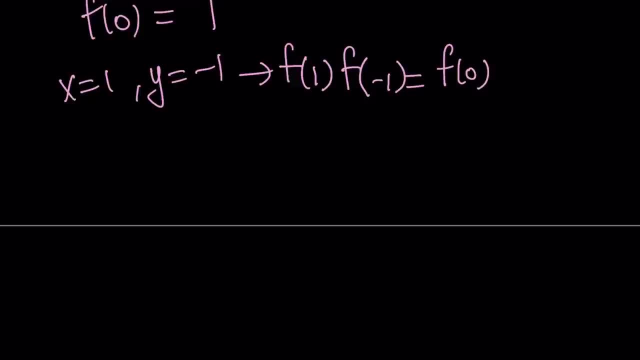 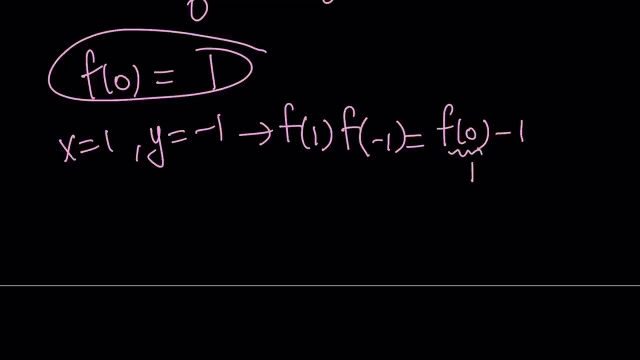 the motivation behind replacing x and y with opposite values, because you're going to get f of zero on the right hand side, And you do know what f of zero is. We know that f of zero is equal to one. So we're going to replace f of zero with one here, And that's going to give us f of one. 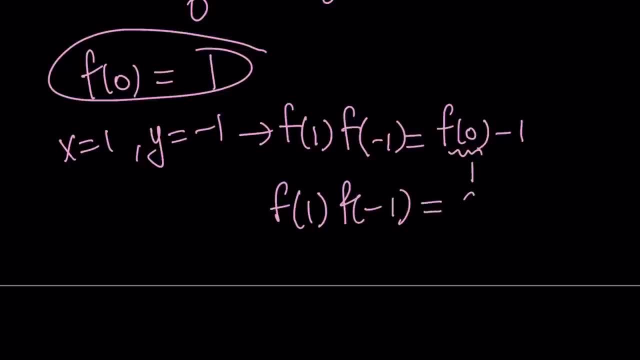 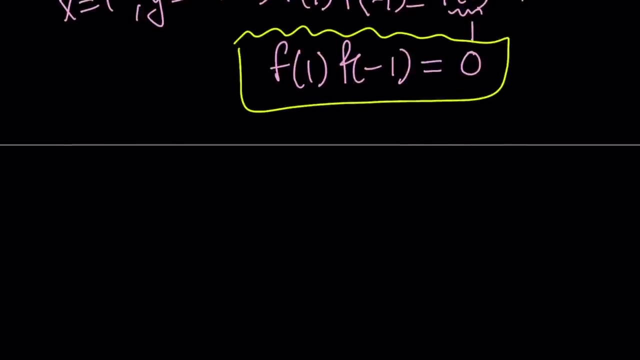 times f of negative one is equal to zero. Awesome, This is a really good finding, Because, again, f of these has to be zero. But do we know which one? No, not really. You can go to the original problem. you can replace x with you know one and one, But that's not going to help us, As you've. 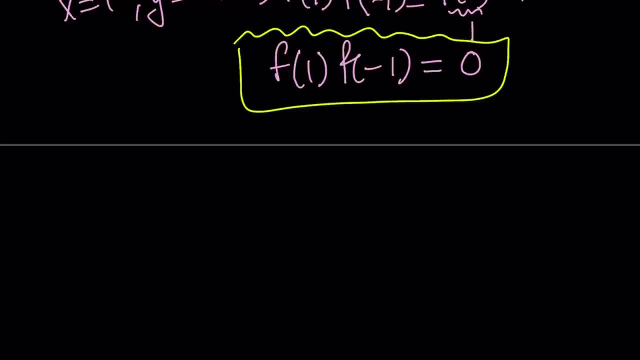 seen before it's, we have to deal with f of two. you can do one and negative one, But we already did that, So it's not going to give us anything additional, Anyway. so here's what we need to do: We have to look at both cases. So, suppose, suppose. 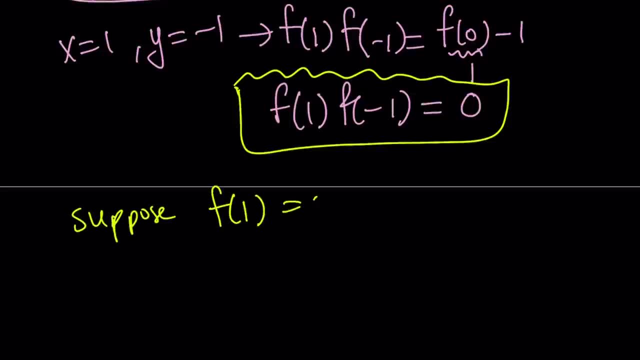 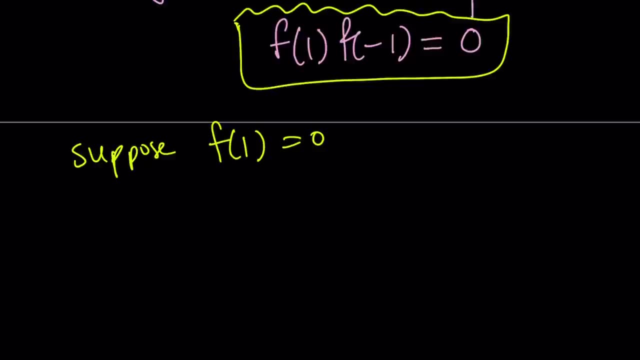 f of one is equal to zero. Now, this is going to give us a solution, And now we're going to look at the second case. Now, if f of one is equal to zero, I'm going to replace x with z minus one. 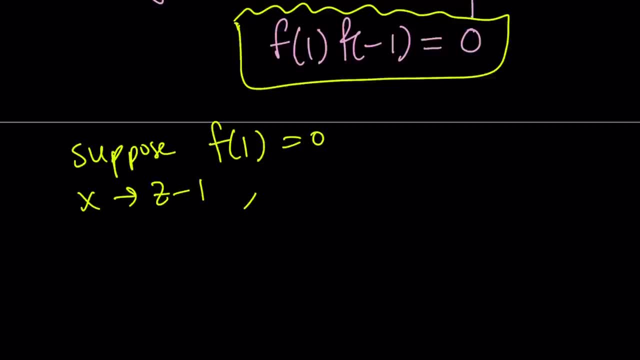 And the reason behind this is I don't want to use y or x again. you could? I mean it doesn't like it's no big deal, But I just want to use a different variable And we can always convert something like f of z to f of x easily, because we can replace z with x- Awesome. 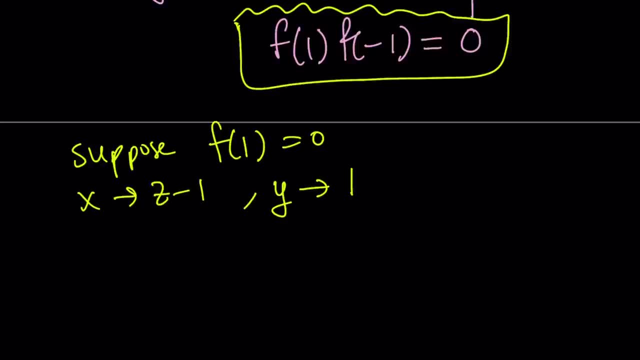 Now in the original problem, remember we have f of x times f of y, So it's going to be f of z minus one times f of y is going to be f of one equals f of. now you add x plus y, you're going to get z. 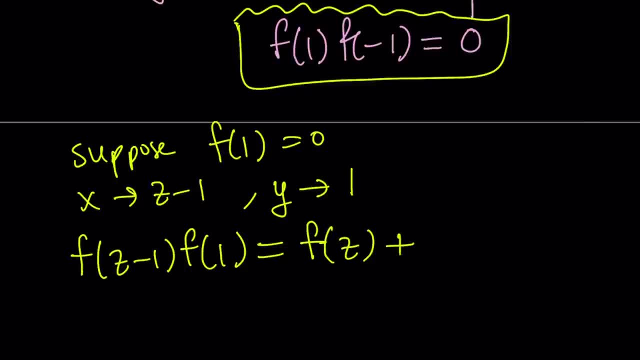 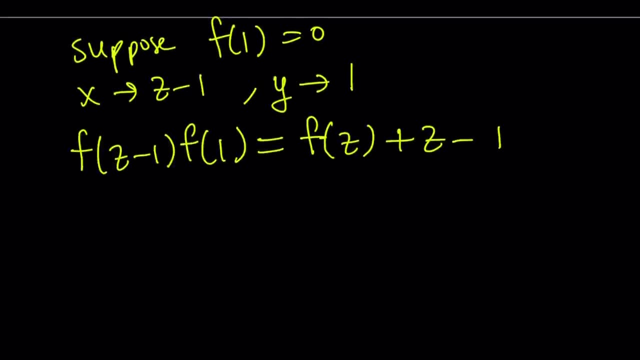 and then plus x, y, which is the product. that's going to be z minus one. Now this is really cool, because f of one is equal to zero. That's what's really cool about it. So now we can replace f of, and that's going to give us zero on the left hand side. Let's go ahead and write the right. 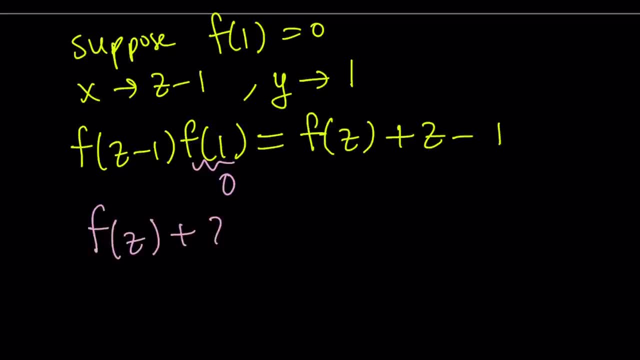 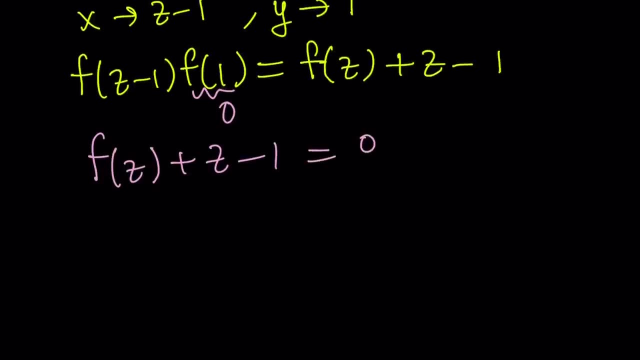 hand side on the left hand side and the left hand side on the right hand side. Okay, I hope that makes sense. So this is going to give us f of z plus z minus one equals zero. Yay, this is beautiful, because this gives us f of z as one minus z, And from here, obviously, we can find f of x by. 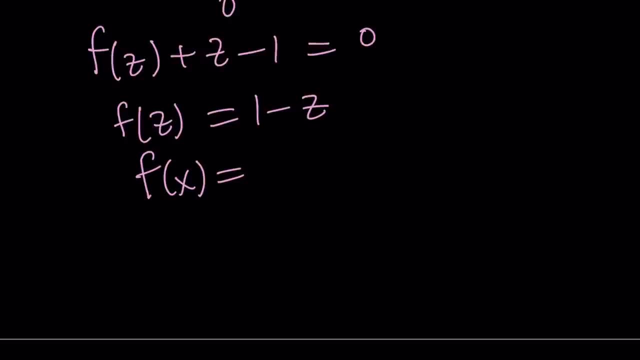 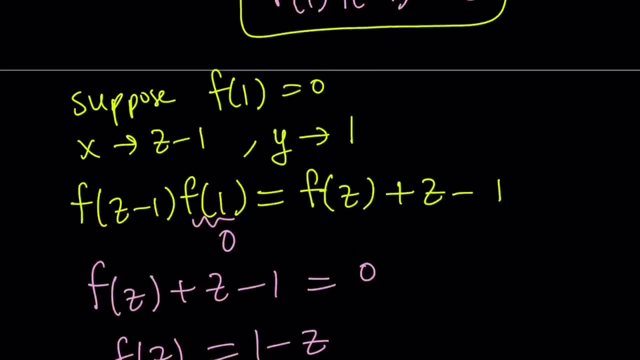 replacing z with x. Don't worry about all these replacements, because these are dummy variables. they're just dummies And we get f of x equals one minus x as a solution, And definitely you can verify that f of one is equal zero. But again, this is. 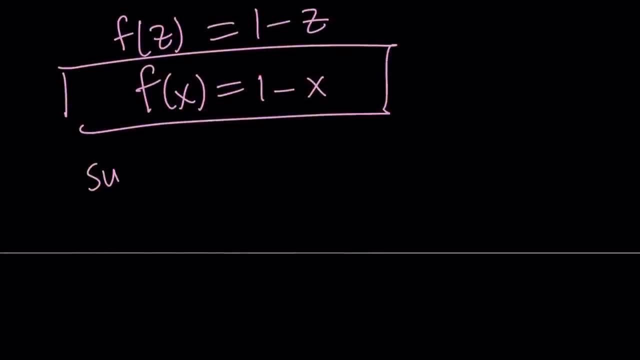 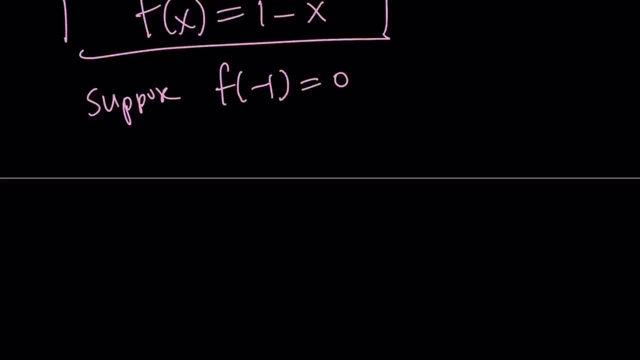 if f of one is equal to zero. Now suppose f of negative one is equal to zero, And let's see if we can find a different solution from here. If f of one or if f of negative one equals zero, then I'm. 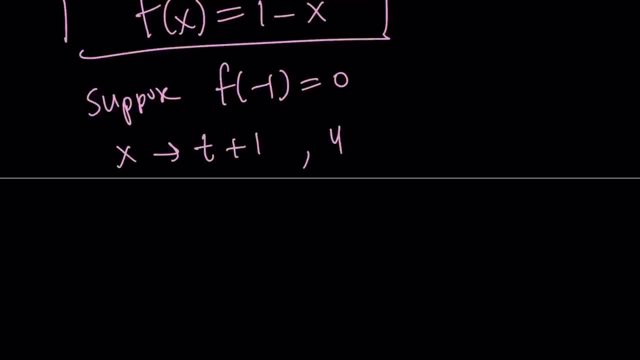 going to replace x with t plus one and y with negative one. And of course there's a motivation behind this, because I want there's some to be a variable like t or z, And I want to take advantage of the fact that f of negative one is. 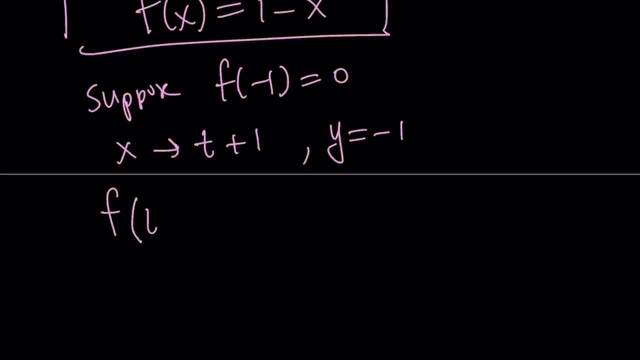 equal to zero. So that's the motivation: f of t plus one multiplied by f of negative one equals f of t plus one minus one, which is t plus t plus one multiplied by negative one. that's going to be negative t minus one. Awesome, But f of negative one is equal to zero, because that was our. 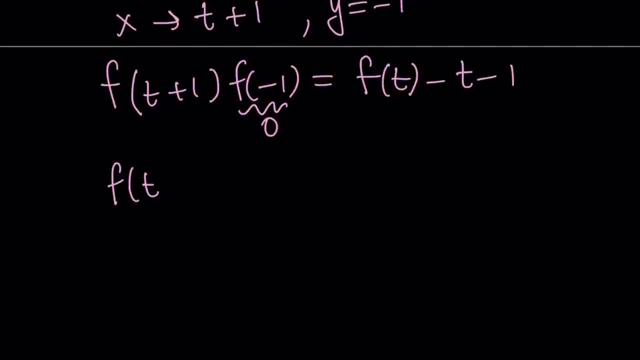 initial assumption: f of t minus t minus one equals zero. And from here we get: f of t is equal to t plus one. And again you can verify that f of negative one is equal to zero. here, if you plug in t equals. 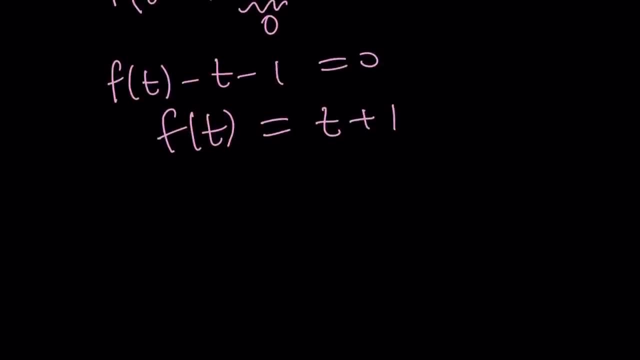 negative one. All right, great. Now what am I going to do? I want to find f of x. Therefore, I can write it as x plus one. So we got two solutions. Basically, one of them was one minus x, the other one is x plus one, And or you can write this: 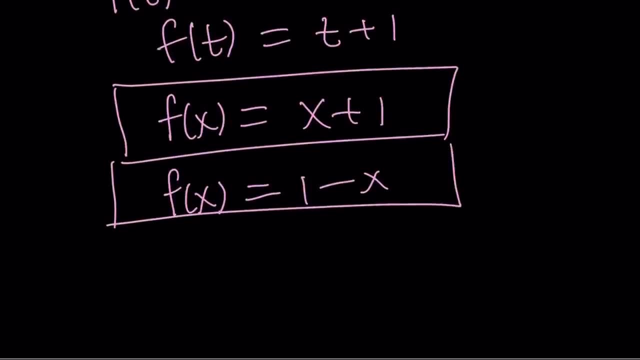 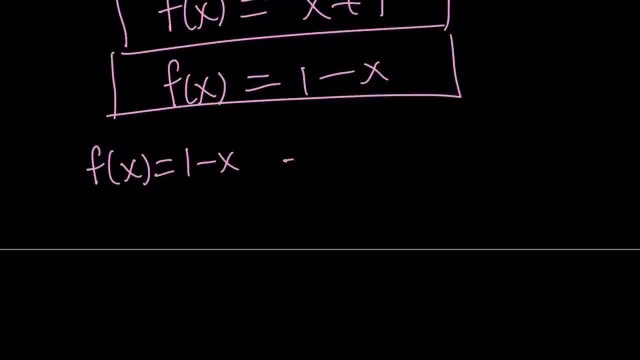 as negative, x plus one, or you can say plus minus, x plus one- our family of solutions. But guess what? if you go ahead and use these values, just kind of plug into the original, you're going to notice that they satisfy the original system as well And there are no other solutions because 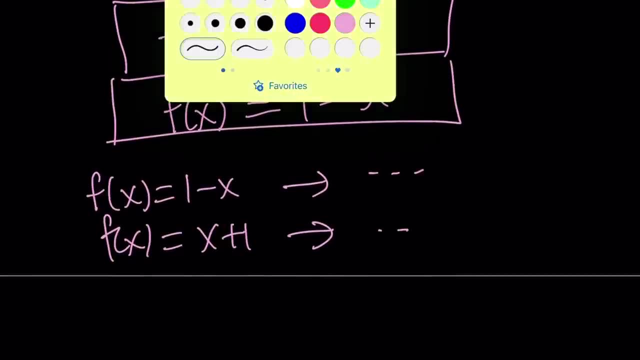 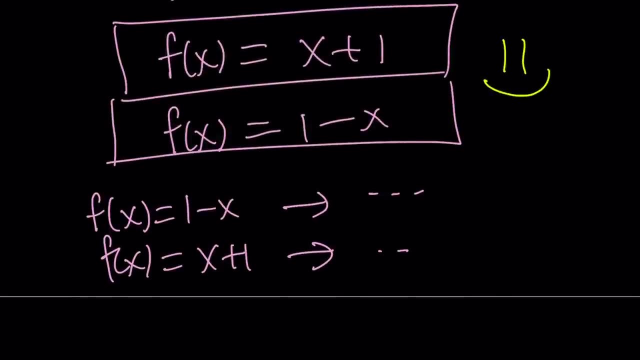 we looked at all the cases, And this brings us to the end of this video. Thank you for watching. I hope you enjoyed it. Please let me know. Don't forget to comment, like and subscribe. I'll see you tomorrow with another video. Until then, Be safe, take care and bye. bye.